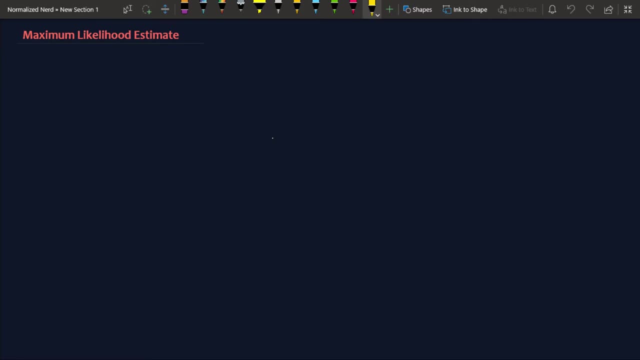 In this video, I'm going to be diving into the mathematical details of maximum likelihood estimate, and I will also show you how you can use this maximum likelihood estimate method to derive different cost functions in machine learning, like the least squares cost function and the binary cross entropy cost function. So this is going to be a mathematically intensive video, So please turn on your math senses. Now, what is maximum likelihood estimate? Well, this is actually a 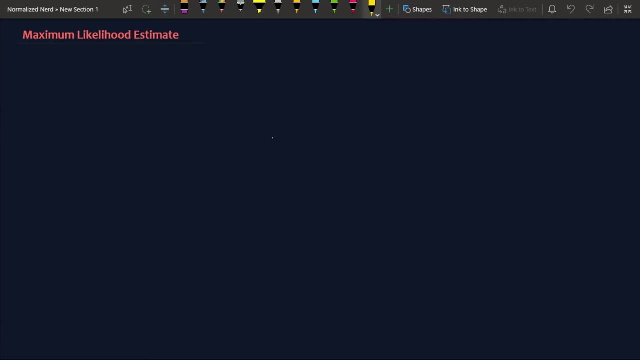 method for determining the parameters of our model. So what the hell are parameters? Well, parameters are those term in the equations of your model which makes it applicable for your particular problem. Now, what does it mean? So let us take an example. Suppose I am taking an example of a linear regression model which we can generally regard as y is. 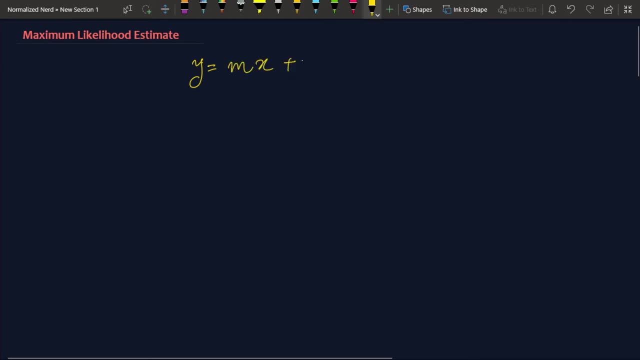 equal to mx plus c. Now, this is a linear regression model and this linear regression model can actually be applicable on many cases like predicting house prices, predicting future values of a commodity, and so on and so forth. Now, what we do? suppose we in our problem, one which is the house price prediction problem, Suppose the prices are distributed. 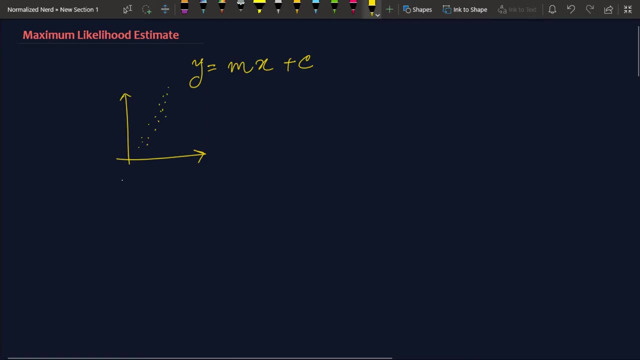 in this manner, We can actually get our final line as this one: Okay, and in another problem, suppose we have to predict the value of a commodity. Now suppose in that case we have the data point like this: Now, in this case you can see that the line will be something like that: Now you can see that both of these lines can be generalized by this formula, but this: 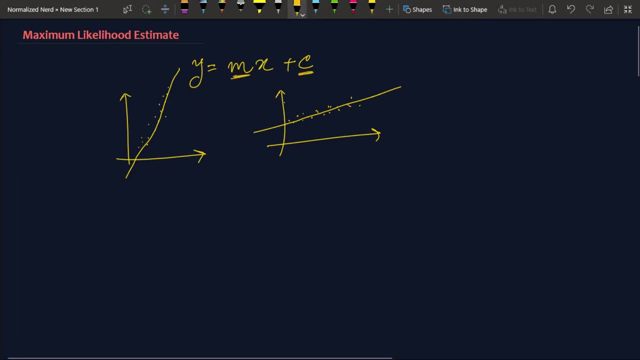 m and c will vary from case 1 to case 2. so this m and c are the values which actually makes our model useful to our particular problems. so this m and c are called the parameters of our model. okay, so i hope the concept of parameters is clear now. now what this method does it actually 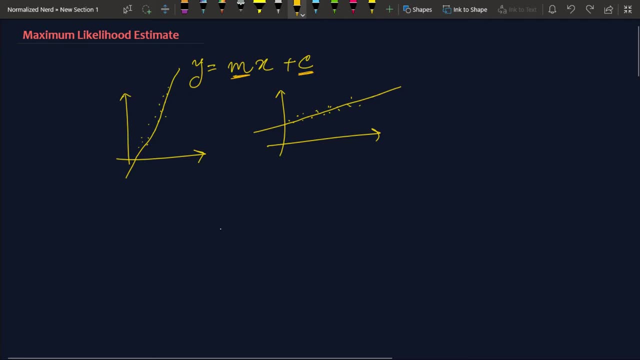 finds the parameters by maximizing the likelihood. now, what is likelihood? well, the likelihood is actually defined as the joint probability of a given data for a set of parameters. now, it is mathematically same as finding the probability of the data, where we know the parameters beforehand. so mathematically, we can write the likelihood of some parameter. 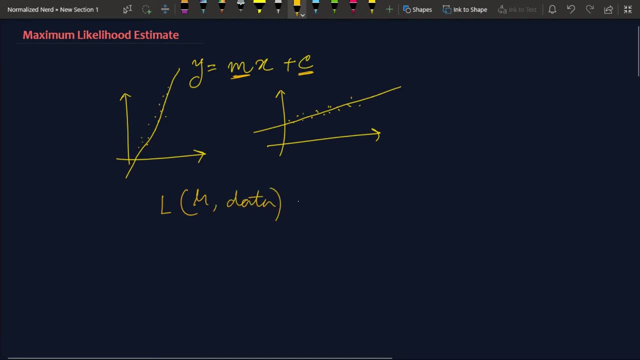 given the probability of the set of parameters. and we can write: the likelihood of the set of parameters, given the data, is actually equal to the probability of the data given the parameters. now, so what's the difference? the mathematically they are exactly the same, but conceptually they. 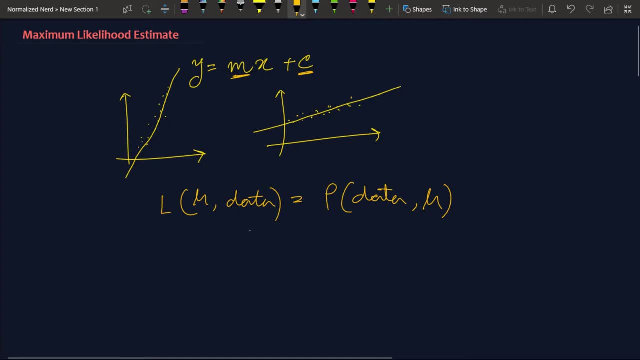 are not well see. in the likelihood case we have the data first and we don't know the original parameters of the data. that is, we actually don't know which distribution is applicable for this data. so we take some dumb Mike Atkins new and we apply Kim to the formula. the probability have the 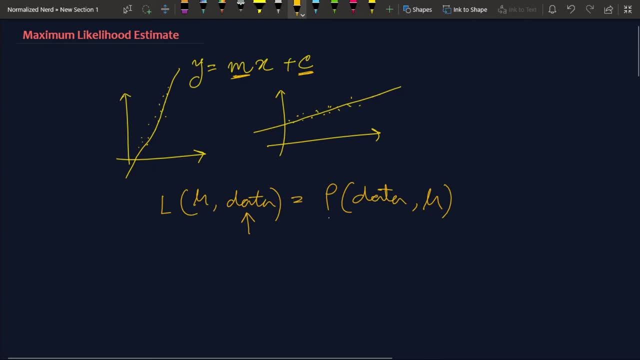 beta flop this set of parameters? why, in case, Obama is violating? we actually know the distribution of the data, that is, we actually know the ship and the parameters of this data and we want to find the probability of some new data. does it go to do that distribution? so we talk. 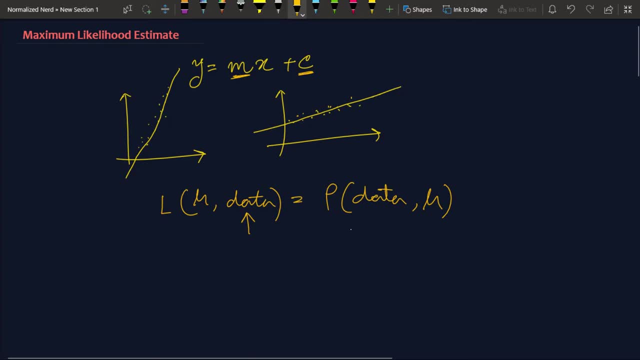 about likelihood. when we have the data first and we talk about probability, know the distribution and the parameters first. So let me give you another example where the things are conceptually different but mathematically same. So let us take an example of an object here. 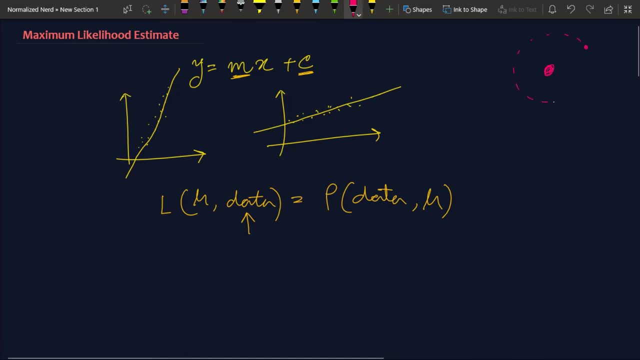 and another small object rotating at a fixed distance. So the radius of this orbit is constant. Now, from our reference frame we can define a force named centripetal force, which is directed towards this. but from the reference frame of this object we can actually define 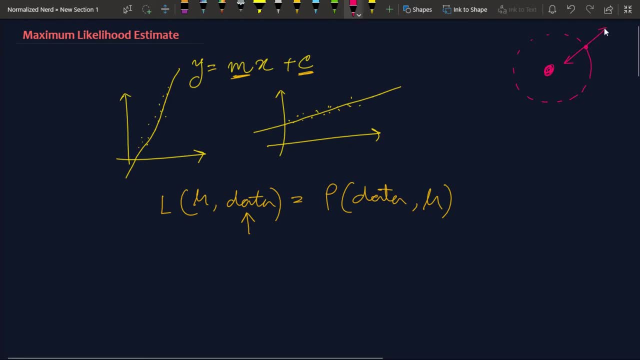 another force, which is called the centrifugal force. Now, conceptually they are different, but the mathematical values are actually the same. So I know that this example is not a very good example for this one, but for sake of the intuition, I just mentioned this that in some cases it happens. 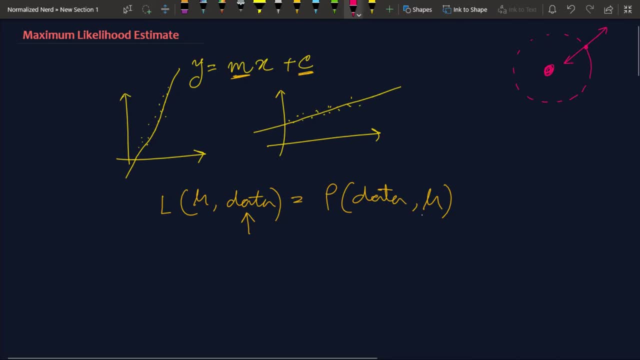 that the things are mathematically the same but conceptually different. So that is the case for likelihood. So I hope the concept of likelihood and the difference between likelihood and probability are clear now. Well, it will be more clear when we take an example. So let us. 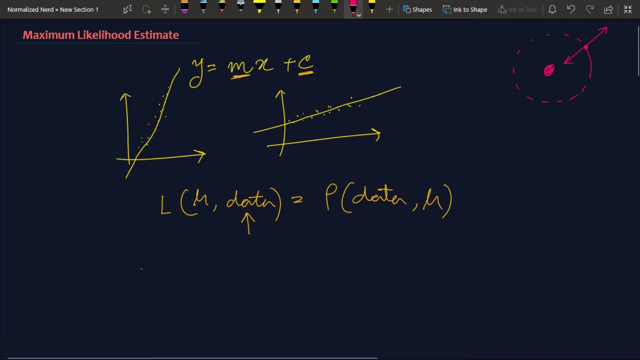 take an example. Suppose we have a data containing the scores of some students in a class in a particular test. Now let me draw the axis containing the scores. So suppose this is 0,, this is 50 and this is 100 and we have n number of students. So we have n number of students and we have n number of. 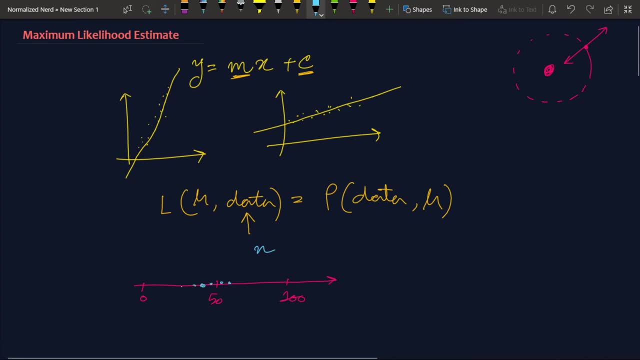 students and the scores of the students are distributed something like this, And we want to know what is the distribution of the scores of the students Now here. in this case, it is actually a good guess to assume that the distribution will follow the normal structure. that is the distribution. 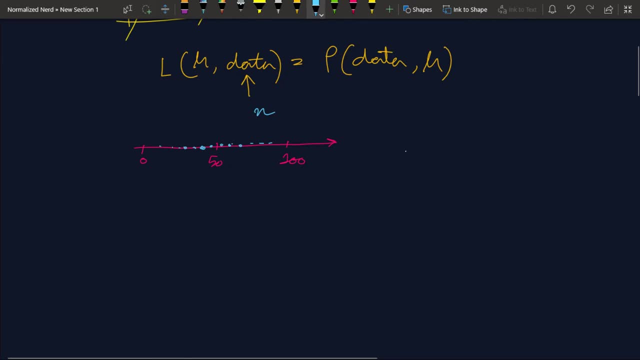 will be a normal distribution. So I am assuming that this distribution is actually normal distribution, with the parameters mu and sigma squared, and mu is the mean and sigma squared is the variance. obviously, And we want to know the likelihood of this mu and sigma, given that our data- and here I am writing the data as x- 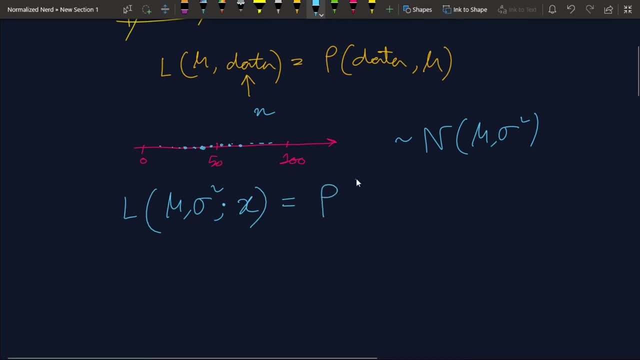 Okay, so mathematically it is same as probability of this data, given that this parameters- Now, in this case, remember that, as I have told earlier that likelihood- is actually the joint probability distribution. So, whenever we calculate the joint probability distribution over a set of values, we 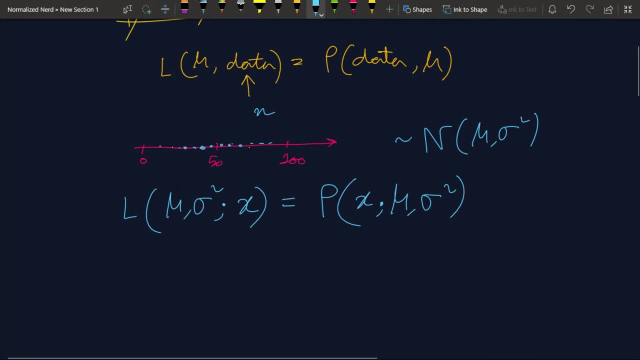 should ideally consider the effect of one point on some other point. But if we consider that, then the complexity of the computation will increase exponentially and we definitely don't want to do that. So, for the sake of simplicity, what we do, we assume that the probability of the distribution is 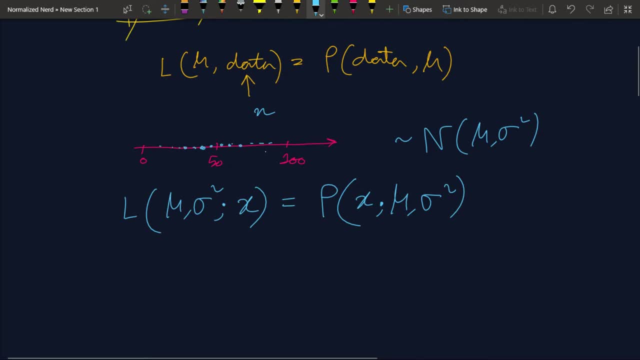 actually independent. We assume that these points are actually independent, That is, we can actually product the probabilities of each of them. So the product will run from i to n. probability of Xi, given the mu and sigma squared, And if you remember the formula for probability in case of: 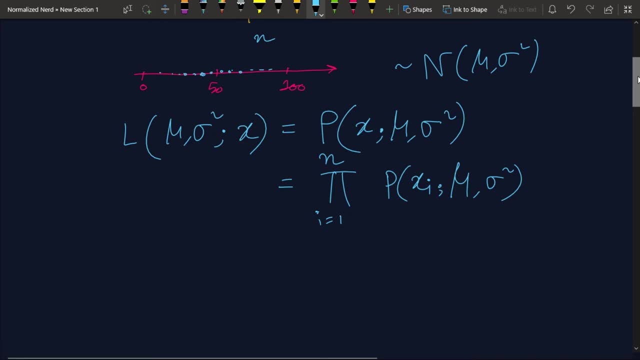 this normal distribution, then you are able to calculate the probability of the distribution. Now, in this case- again, remember that these points are actually independent. They are actually independent- Then it is simply as 1 over sigma root over 2 pi, and here we will have e to the power. 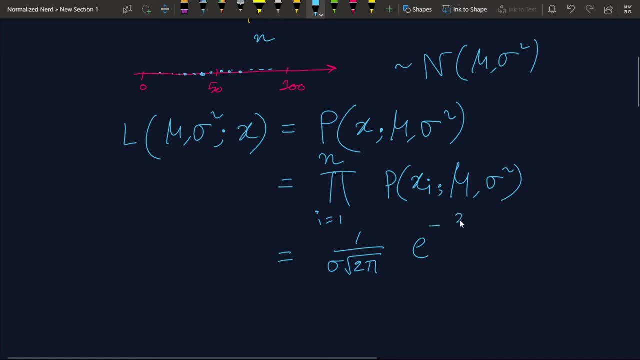 minus, say xi, minus mu squared, divided by 2 sigma squared, and the product: okay. So by maximizing this likelihood, we are actually going to find this. parameters: mu and sigma. So what we do here, We go one step forward and we actually take the log likelihood in this case, because it 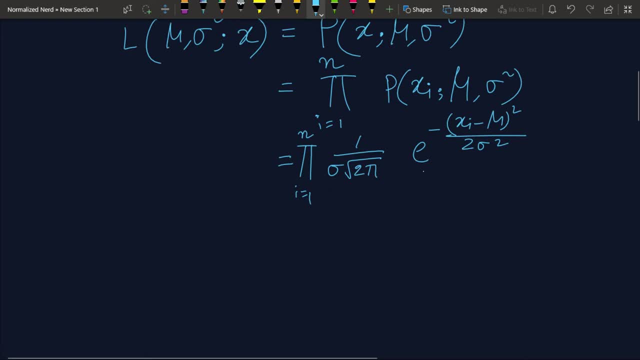 is easier to work with summations in case of a maximization problem than to work with this product. So by taking the logarithm we will gonna have log. well, obviously, the base of this log will be natural, that is e. So log L will be the summation of this one minus. 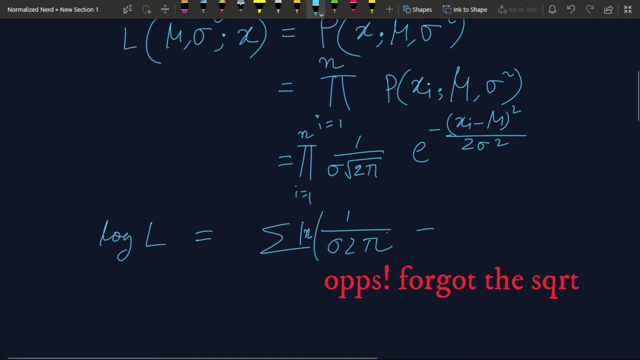 Here will be log xi minus mu, 2, by sigma squared and this squared, and obviously this will run from 1 to n. I hope the concept of maximum likelihood estimation is quite clear now, and now I am going to show you how you can use this concept to derive some of the most famous cost functions in. 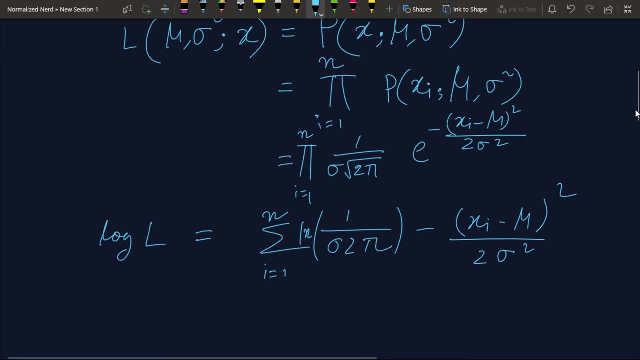 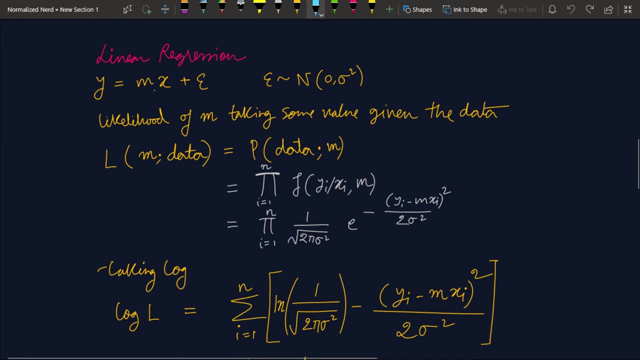 machine learning models. So the first thing I am going to show you is gonna be the linear regression cost function. that is the least square cost function, So let's dive into that. So here I am taking the most simple linear regression model that we can have. that is: 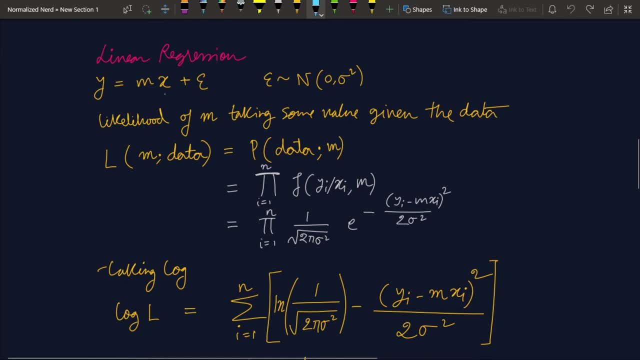 y is equal to mx. Now, I am not taking the intercept term, that is, c here, but if you include that, the mathematics will be more or less the same. Now here we need to do a trick, that is, we have to introduce an error term that I have. 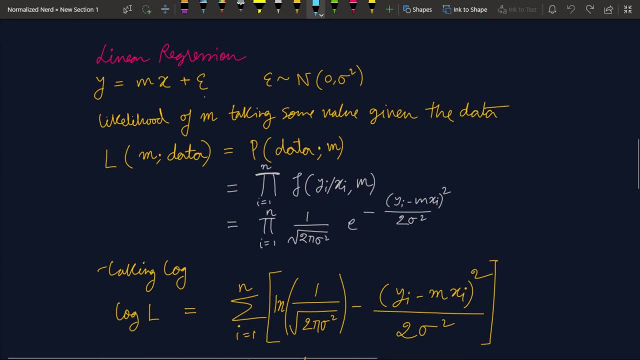 denoted here as epsilon. Now, what does it mean? Well, it means that the error that is generated by our model follows a normal distribution. that too, with mean 0 and variance sigma squared. So this will actually help us to apply the maximum likelihood estimate method. 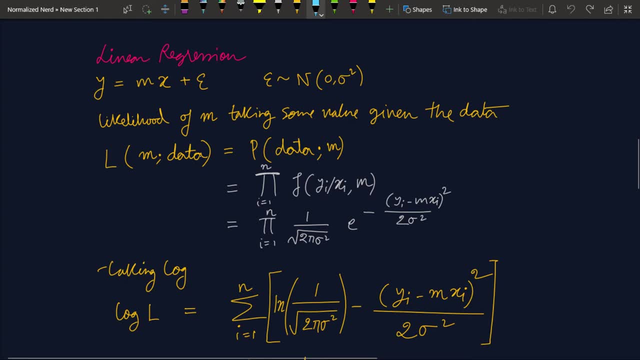 So we are gonna find out the likelihood of our data, Assuming that we have some parameter m, and which is exactly same as the probability of the data given the parameter m. So it will be equal to the product of this thing. So, as I have mentioned earlier that we do not consider the effect of one data point, 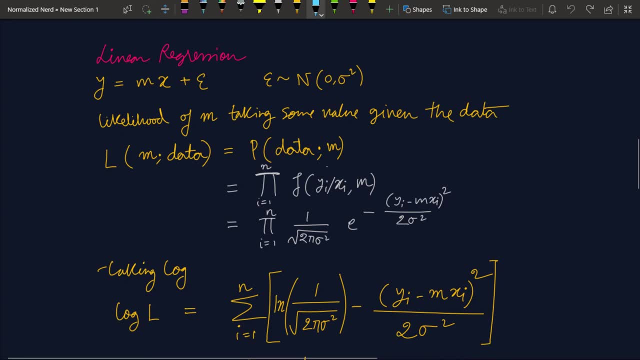 on the other. That's why we can use the product rule here And by using the same formula For normal distribution. we have this thing Now. again, as I have mentioned, we generally take the log of this likelihood, So we want to maximize this logarithm of this likelihood. 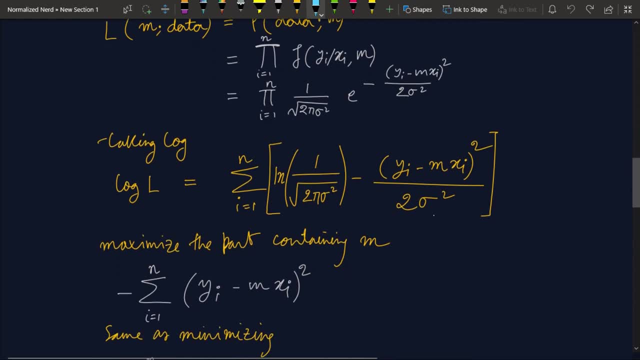 So after applying the log, we have this big thing Now. remember that we only want to find the value of m, So to maximize this part is same as maximizing Only this portion, Alright, and you can see that we have a negative sign here. 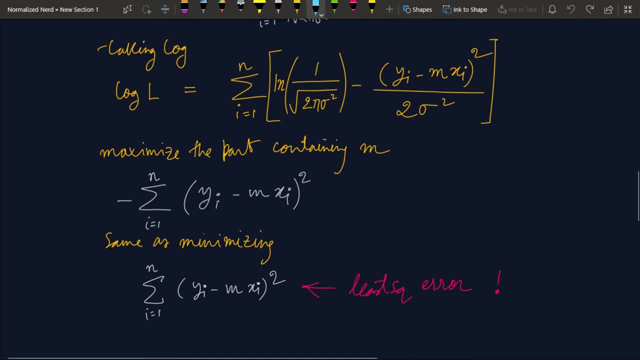 So we can just omit this negative sign, So we can say that maximizing this is same as minimizing this one. And voila, this is actually the least squared error function that we use in linear regression in machine learning. So isn't that amazing that, following some totally statistical tool, 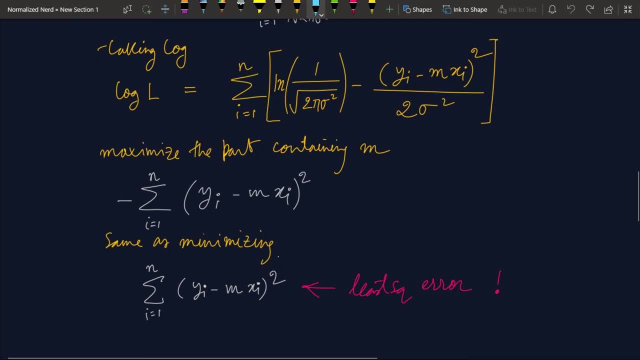 We are arriving at a cost function that is used in machine learning, So I hope the application of maximum likelihood estimate in linear regression is quite clear now, And let's move on to the logistic regression and the binary cost entropy cost function. Okay, Okay. 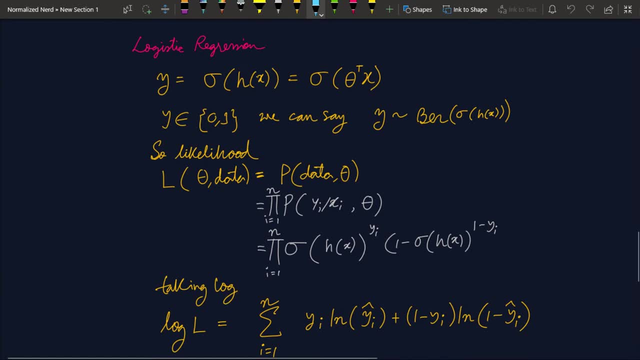 So So we have logistic regression and the general model is as follows: y is equal to well. I hope you know this function here. This is actually denoting the sigmoid function by the alphabet sigma, and the h of x is actually some linear function. Now please be attentive here. 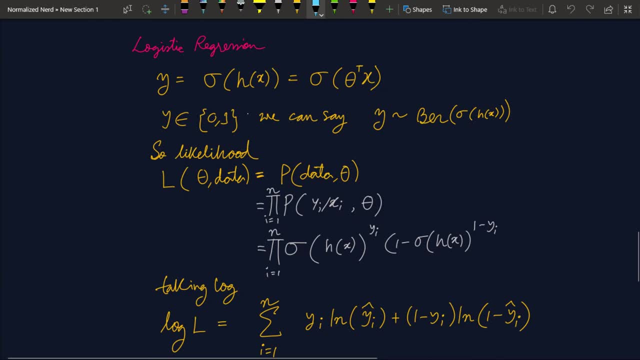 So what does our logistic regression outputs? Well, it outputs a number that can be either zero or one. Well, actually, we need to use a condition here. If the output of this sigmoid function is less than or equal to half, we say that the class is zero, and if it is greater than half, then we say the class is one. 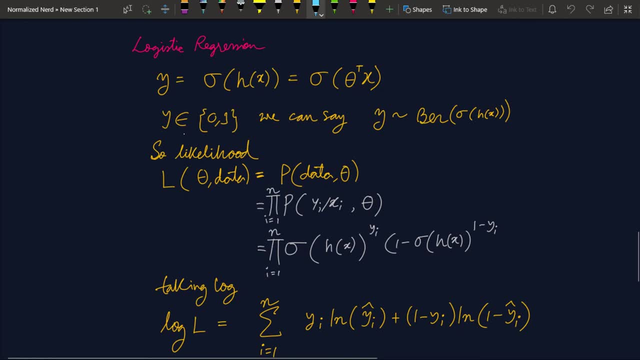 So generally. So basically, our model, after doing the condition, will output one number, zero or one. So we can say that y follows a Bernoulli's distribution with this probability. Now, what is a Bernoulli's distribution? Well, A Bernoulli's distribution is actually a distribution where we have only two values. 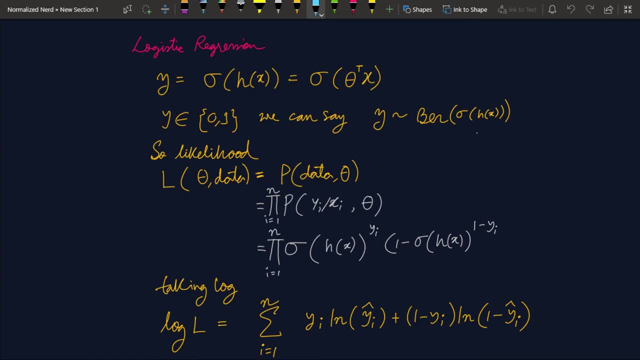 and this experiment is actually called Bernoulli's trials, and in each trial only two possible outcomes are there: zero or one. Okay, Now the distribution looks something like this: Suppose these are the values here, And suppose this is a value for zero. 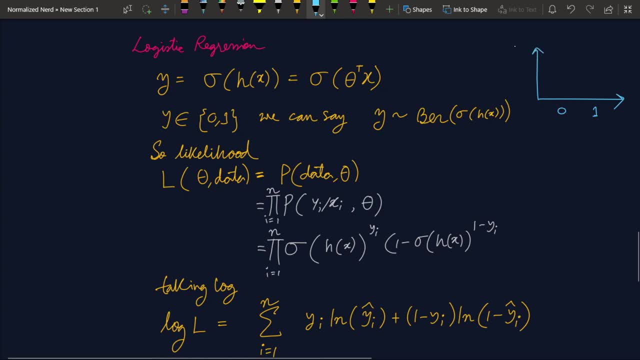 This is a value for one, And suppose this axis represents the probability and the probability of outcome. zero is a fixed one here and the outcome one is fixed one here, And remember, and this one actually represents the probability of the class one. Okay, So if we say Bernoulli, point six: 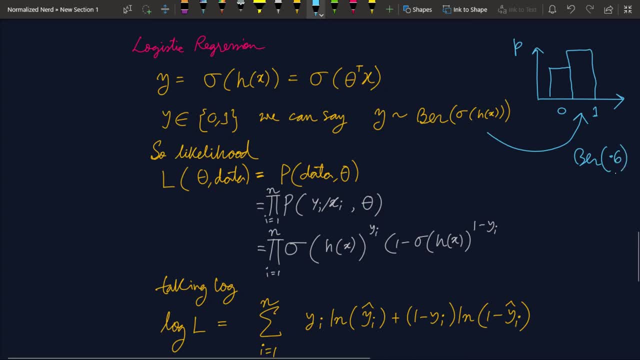 That means This: There is a 60% chance that our Bernoulli's experiment will outcome one and there is a 40% chance that it will outcome zero. Okay, So now we want to find the likelihood as the previous method.